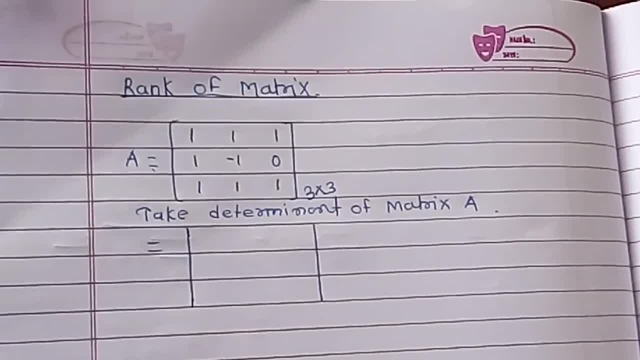 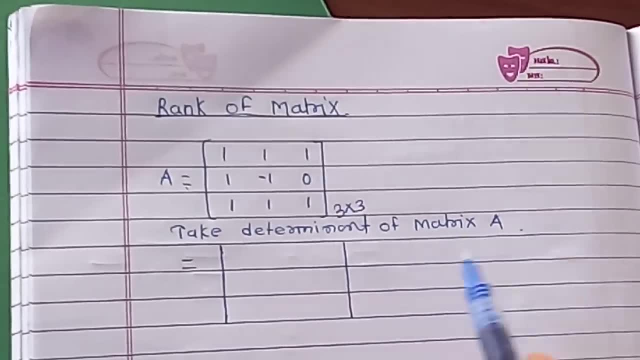 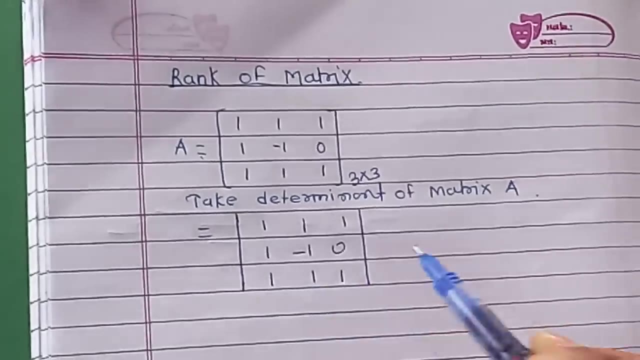 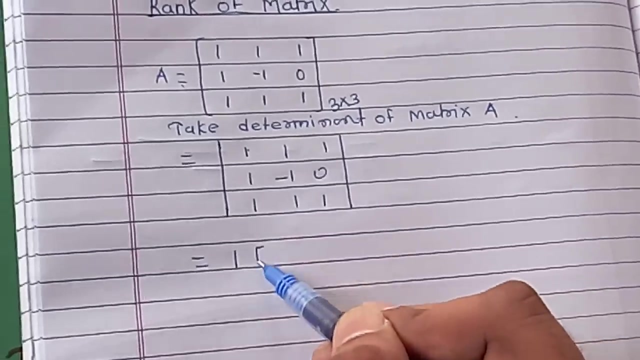 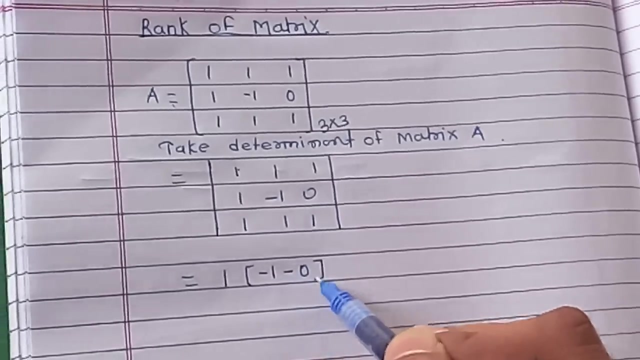 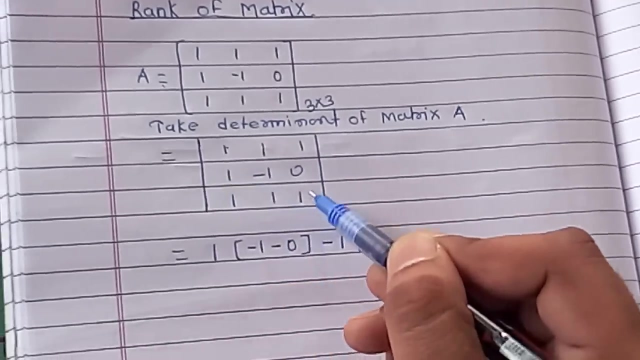 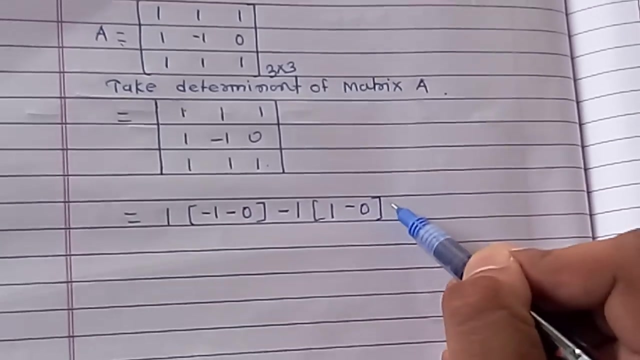 matrix. it is the very easiest and the simple, simplest method in that method. first we have to take the determinant of the matrix a. it is one we have to find out. the determinant of this is one right multiply with minus one. one minus one minus zero. second column: minus one multiply with this: one minus 0 plus 1. 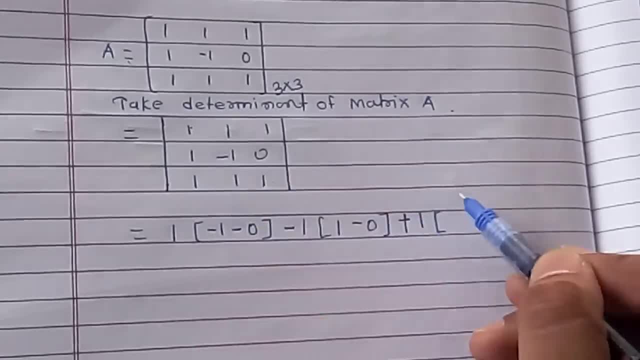 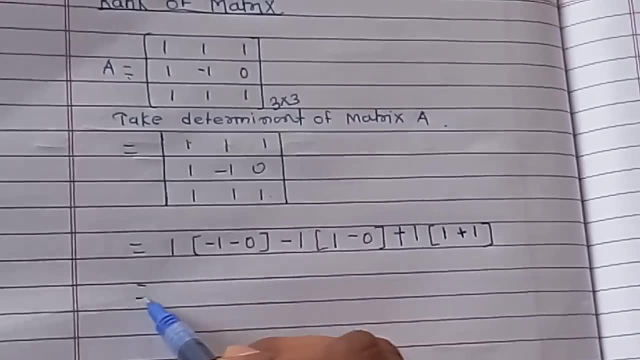 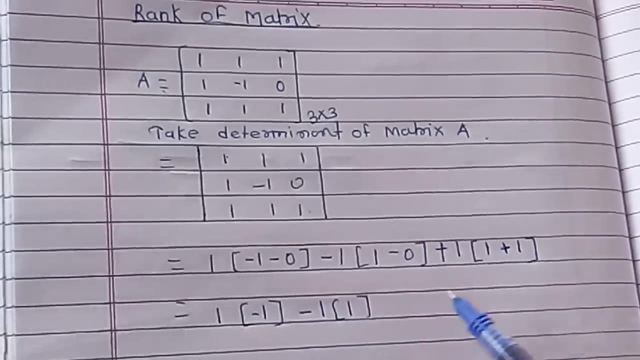 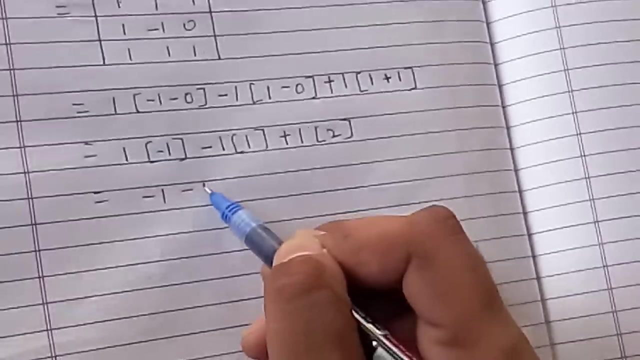 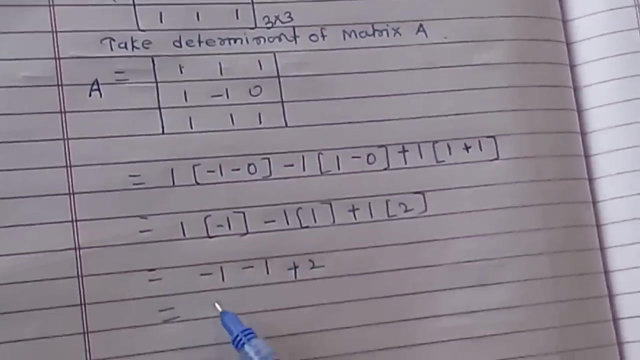 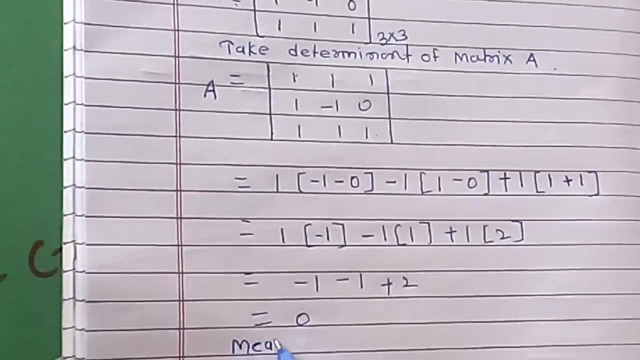 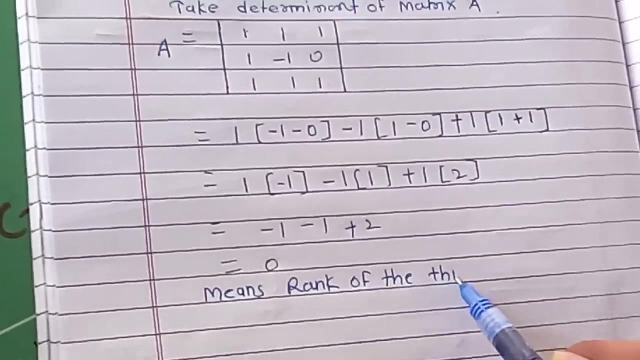 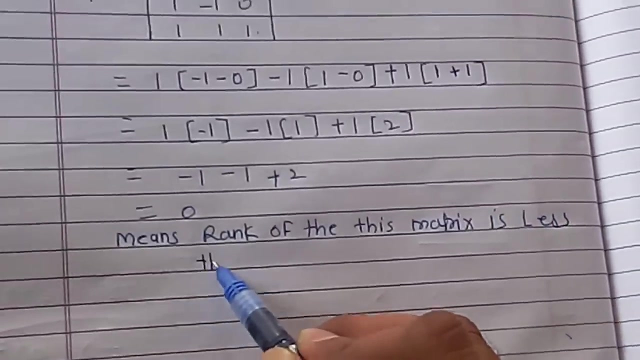 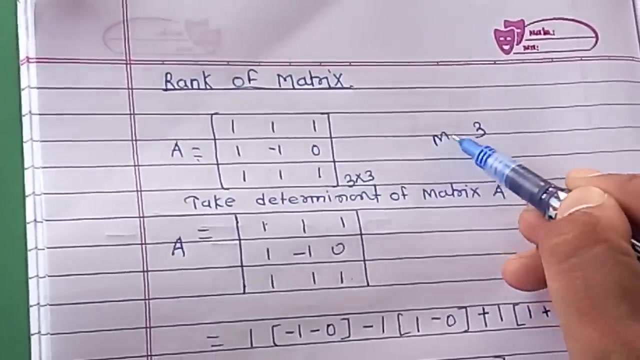 multiply with this: minus minus plus one. one minus one minus 11 plus one. the determinant of this matrix a is 0. meaning of that is that the rank of the matrix means rank of the. this matrix is less than 3 because the maximum rank of this matrix is 3 and minimum whatever. 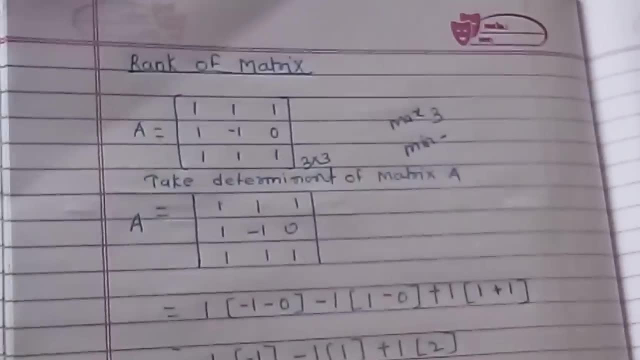 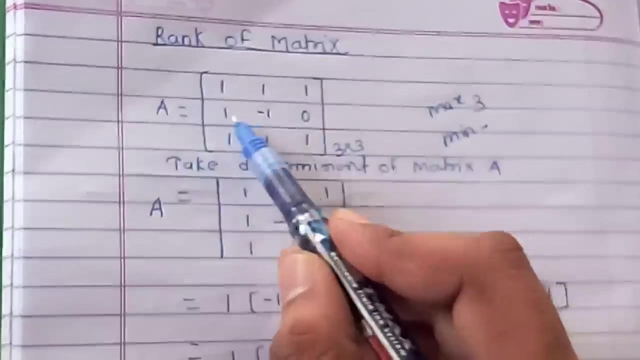 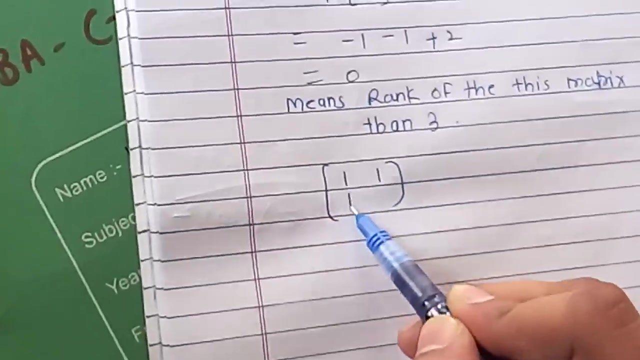 it may be, which we will get. for that purpose, we have to find out. we have to take 2 by 2 matrix. now we have to assume that 2 by 2 matrix like this: 1, 1, 1 minus 1. then we have to find out.